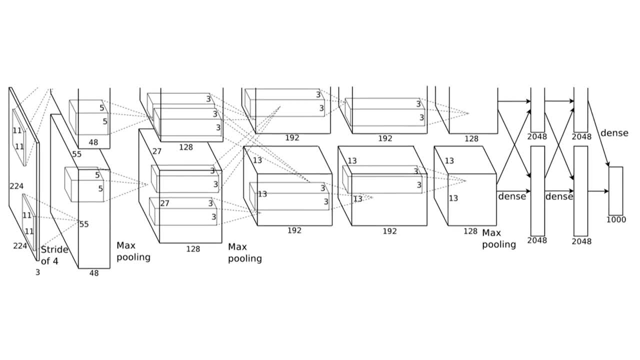 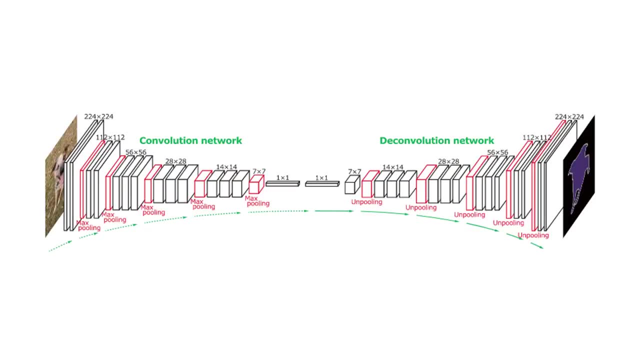 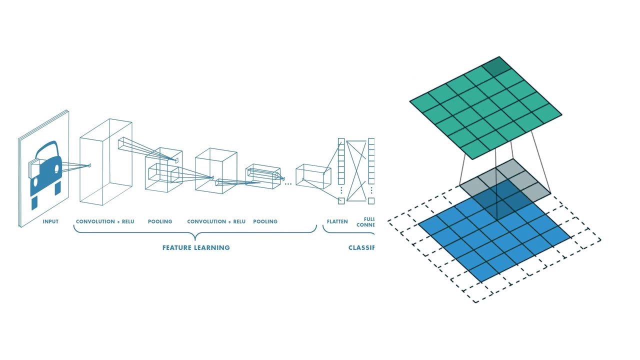 if you've ever looked at a network architecture in a research paper, like this one or this one or this one, or you get the point. Now, if you really want, you can take the 2d animations and the 3d still shots from the research papers and combine them together in your mind. 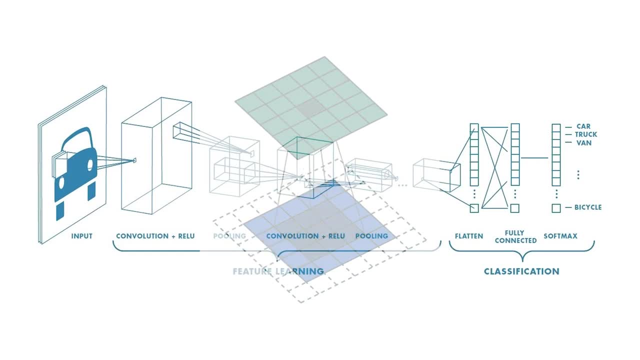 And some people might be fine with this, But I'm creating an introductory course on convolution And I don't want to give my students different ideas about how to do it, So I'm going to give them different pieces of the concept to put together in their head. I just want to show. 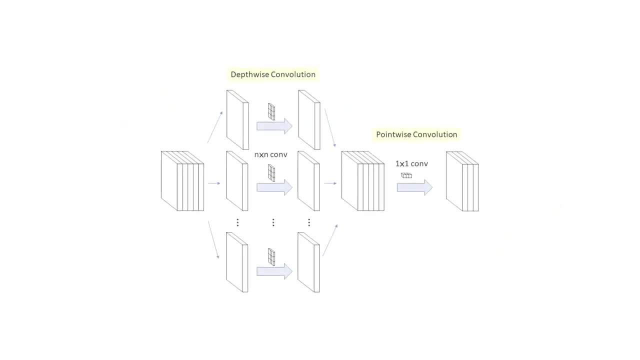 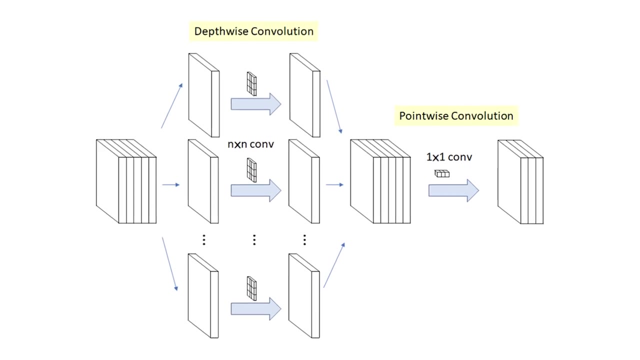 them the end result? And on top of that, how am I supposed to explain more advanced concepts like depthwise separable convolution? I don't want to try and paint a mental video with words and pictures. I just want to show the video. I looked around for alternatives, but they were all wrong. 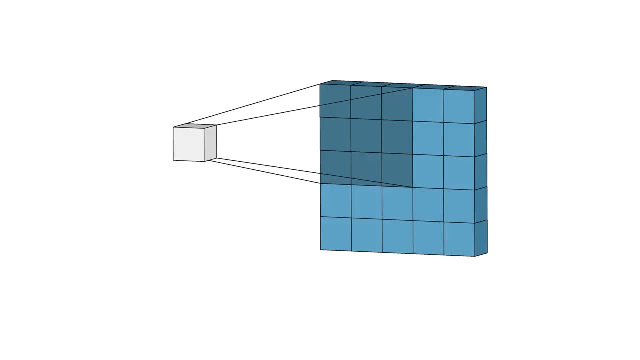 in their own special ways. This one turns the input and output units into 3d cubes rather than squares, which is nice, But it doesn't change anything, So I'm going to show you how to do it. This one does a nice job of showing the filter, but everything is still 2d and it's not animated. 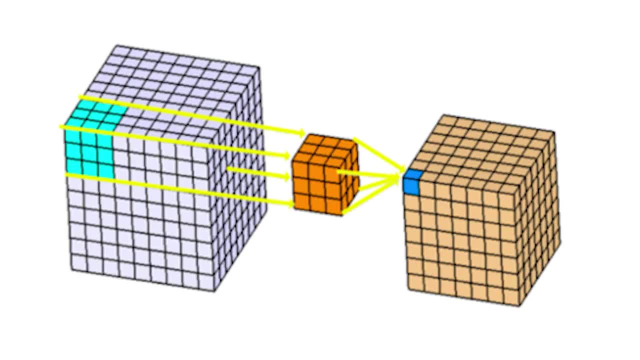 This one looks close right, Except that it's for a 3d convolution, not a 2d convolution. That's why the filter isn't the right size. This one here is pretty close. The filters aren't their true shape. 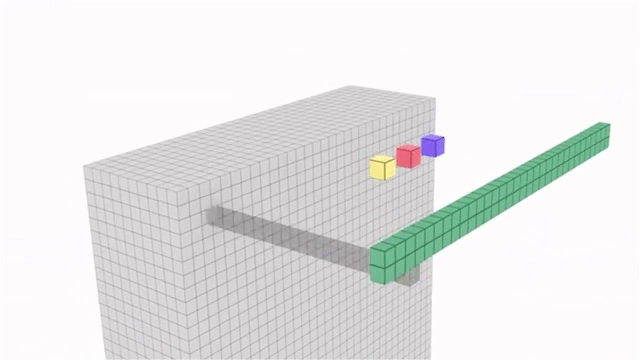 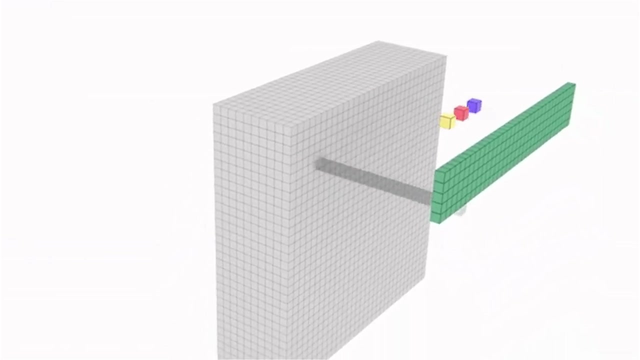 but I could probably live with that. However, I'd prefer a three by three filter so the viewers don't have to guess how the 1x1 generalizes to larger filters. Also, you can see the interaction between the filter window and the outputs appearance as a little awkward. And finally, the camera motion. 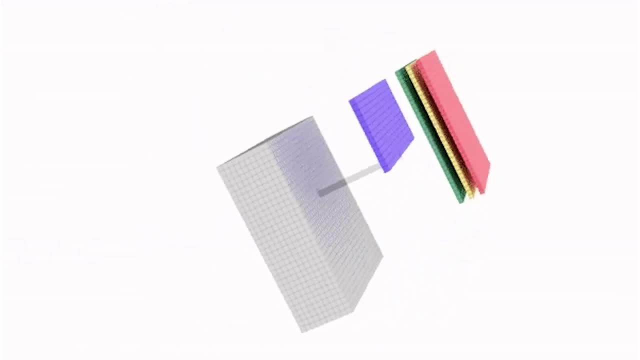 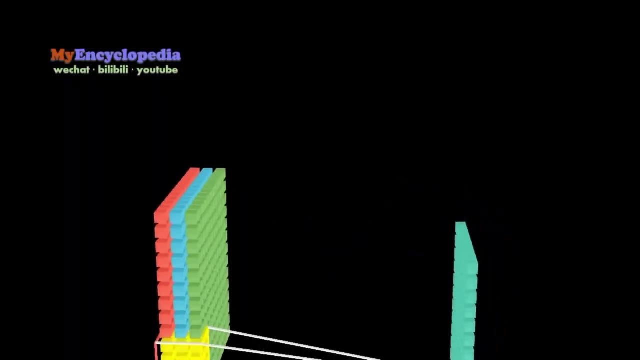 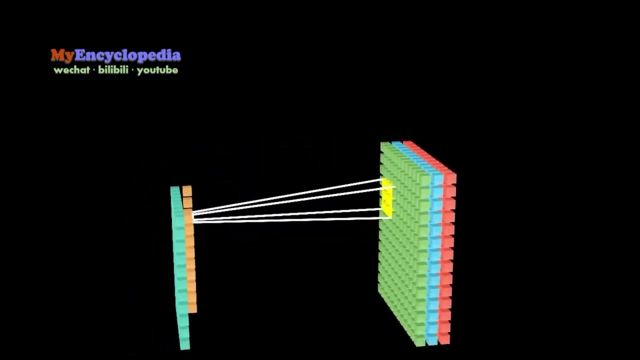 causing the world to flip around is a dealbreaker. I'm not trying to give anyone motion sickness here. Here's my favorite. It's a relatively recent animation that shows a 3d input and actually makes a 3d output, But without displaying the filters. it's not obvious why the output is 3d. 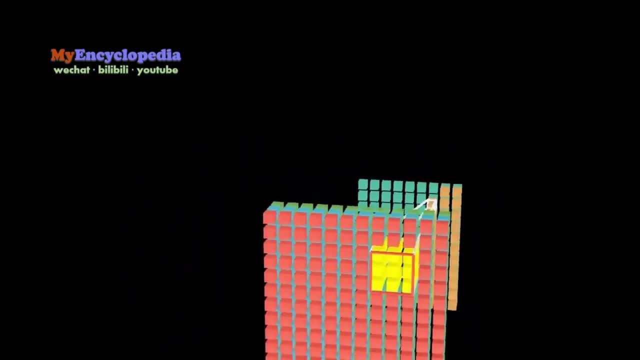 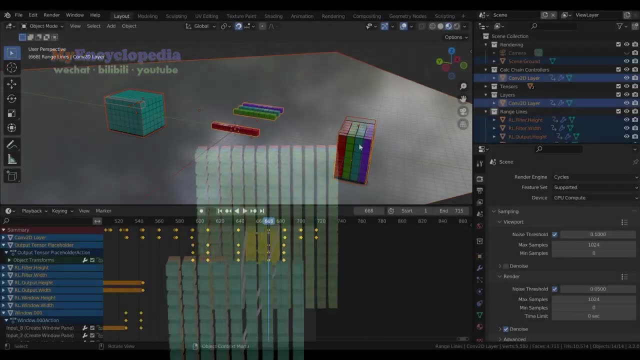 And although the camera movement isn't as bad as the last one, I'd still rather have it be stationary, And those were the best that I could find, So ultimately I decided that if I wanted this done right, I'd have to do it myself.